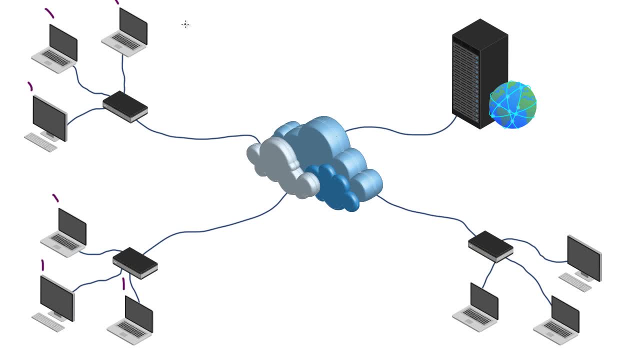 The IP address that you have is actually broken up into two parts, and the reason for this is because the internet is not one big network. The internet is a network of networks. I'm going to say that one more time. The internet is a network of networks. So we have one network over here. This is, you know, some college and this is just some apartment, and this might be an entire country that just got internet for the first time. All of these networks are connected to one network. 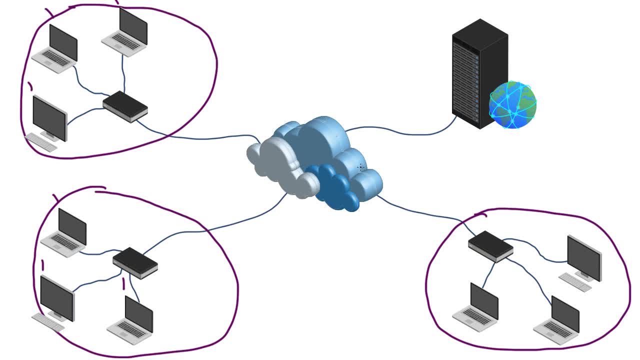 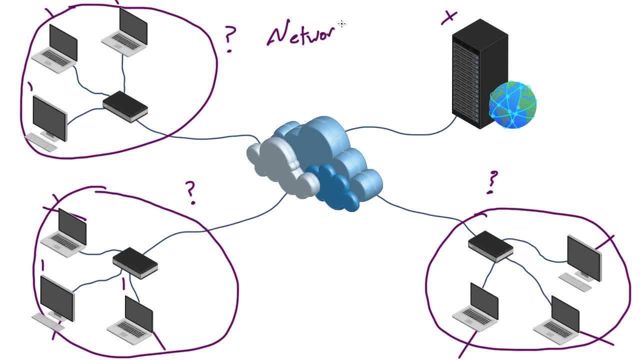 network ID. I'll write these down: network ID and the host ID. so if you can read my handwriting, that's the two pieces of information that we need whenever trying to send or receive data: what network you belong to and what is your host ID. was your individual computers identification or IP address? so way back. 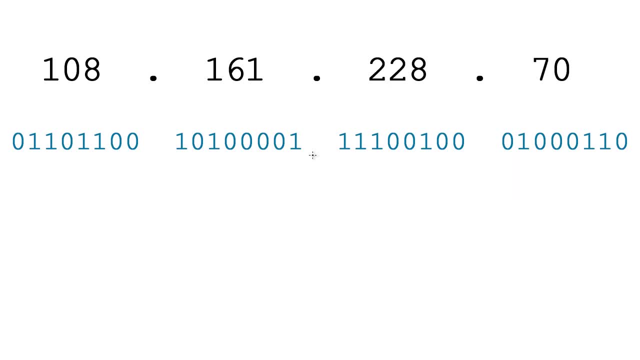 when, whenever they're first designing the IP addressing system, what they did? I don't know what they were doing, probably rollerblading around and smoking weed and doing the disco, whatever the heck they did back then they were looking at this thing and thought, okay, we have 32 bits to work. 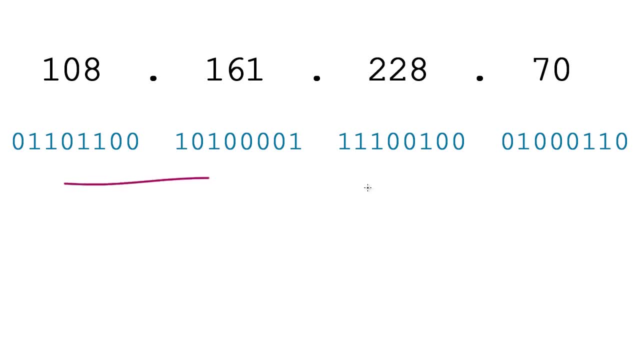 with, and we need to break this up in such a way where part of it is for the network and part of it can be used to identify the host. so how are we gonna do this? well, one brilliant guy probably took a puff on his little joint and was 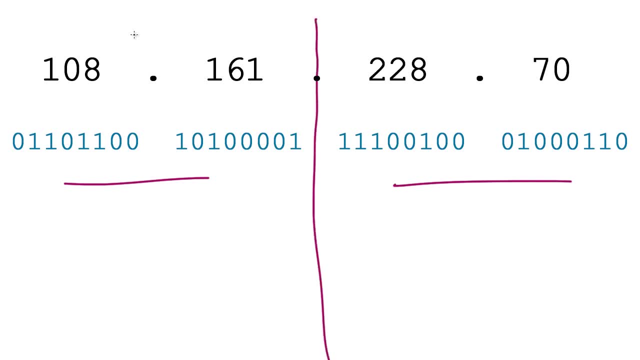 like. you know what, man? why don't we just split it right down the center? this part of the IP dress can be for the network and this part can be for the host. now, whenever we have eight plus eight bits, that's 16 bits, and if we do,